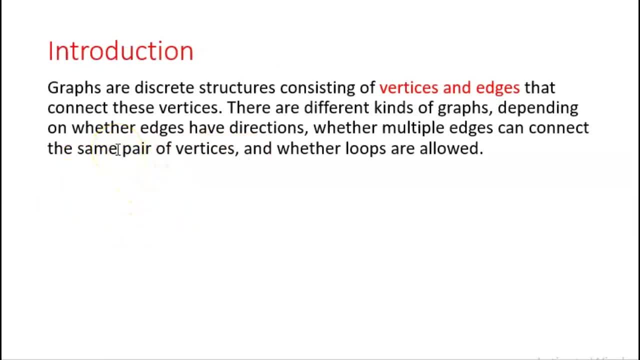 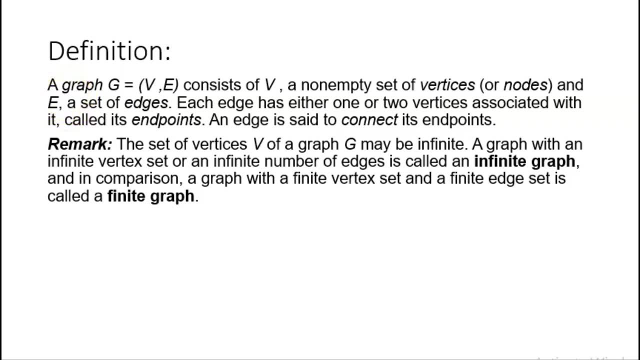 Now be clear about the definition of a graph. So when I talk about a graph, a graph contains two things. So let us look at the definition first. A graph g is equal to v. comma. e consists of v a- non-empty. 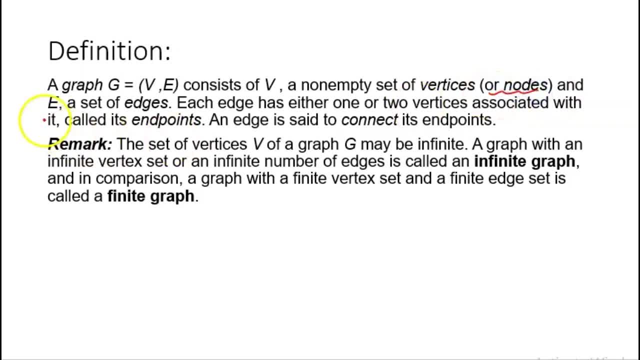 But we can also talk about a set of vertices, which we called as nodes, and E is a set of edges. Each edge has either one or two vertices with it, which is called its end point, And the edge is said to connect its point. There is an important remark which you should be clear about: The set of vertices v of a graph, g may be infinite. A graph with an in infinite vertex 되면 useless, odd, impossible to know. for you, point 1 is bone integral and grade 1 is outside 0 and b is in root constant. 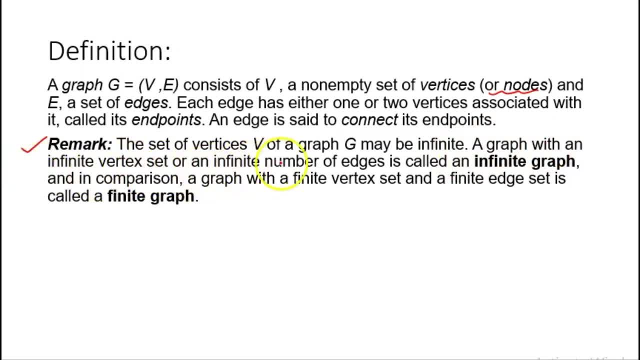 a French definition for this. This word has usual meanings for non-並hing, for smaller vertex set or an infinite number of edges is called an infinite graph, and a graph with finite vertex set and a finite edge set is called a finite graph. in this course we will focus more 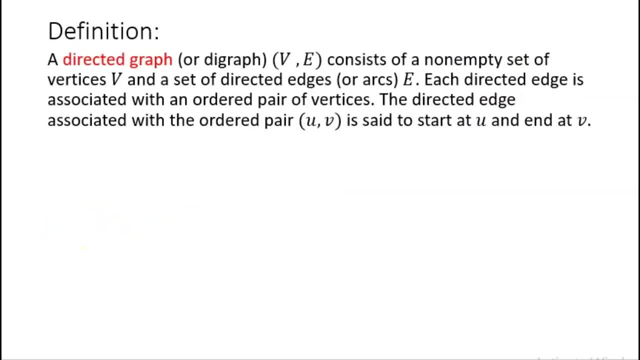 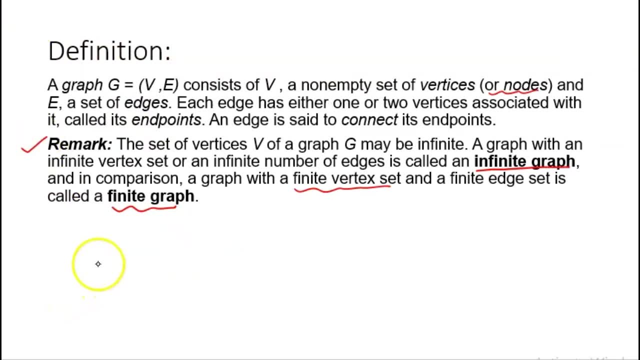 on the finite graphs right now. when i'm talking about graphs, let us understand it through some examples. so suppose, as you have just looked at the definition, that it contains a set of vertices which is non-empty. so i have four vertices here: v1, v2, v3 and v4, and we can join them. so if i'm 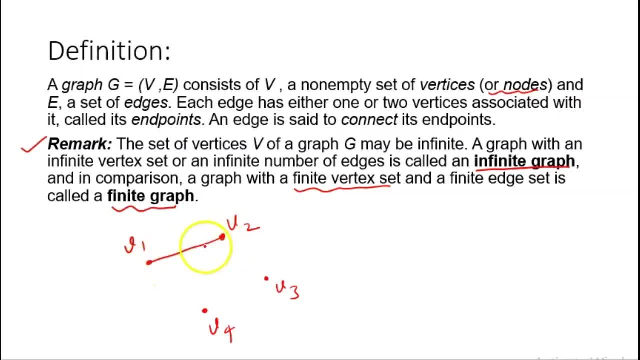 joining v1 and v2. this line is being used to join v1 and v2 and this line is called the edge between the vertices. so if i have a set of vertices, i am joining v1 and v2 and this line is being used to join v1 and v2, and this line is called the edge between the vertices. so if i am 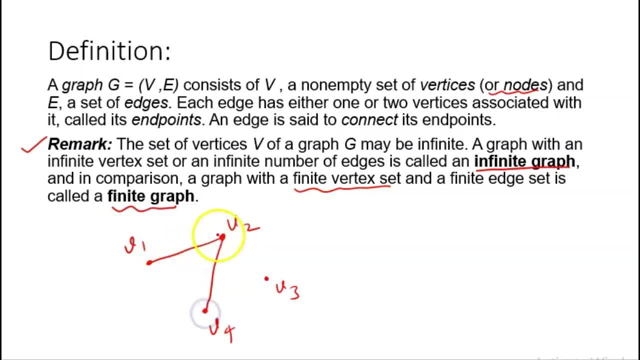 the vertex v1 and v2. similarly, we can join v2 and v4. we can join another edge. we can draw another edge with between v3 and v4. we can join an edge between v1 and v3. so this structure that I have just drawn is known as graph and it has 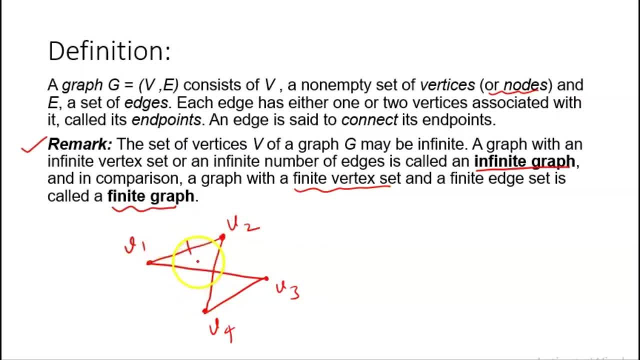 four vertices and you can see it has one, two, three and four, so four edges are also there. so this is an example of a finite graph with four number of vertices and four number of edges. one thing that you have noticed that when I am drawing the edge between v1 and v2, we have not associated any direction like 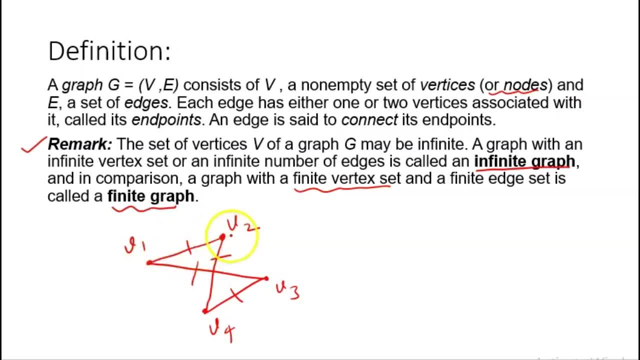 there is no sense of direction, like whether we are moving from v1 to v2 or v2 to v1. so this is an example of something called as undirected graph and we are going to look at the- you know different terminology associated with undirected graph in the. 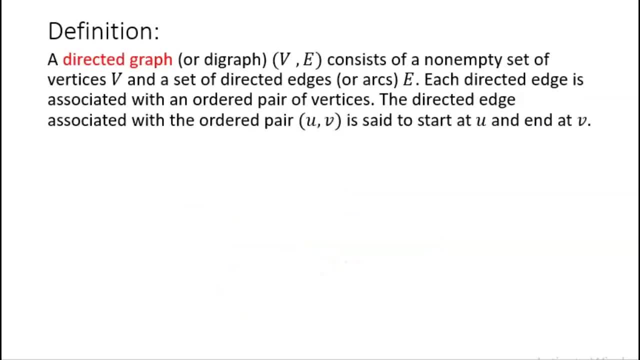 next slides. so if I have talked about undirected graph, there should be something called a directed graph as well. and in directed graph what happens? that there is a sense of direction associated with different vertices, like here we have, suppose. take. let me take v1, v2. 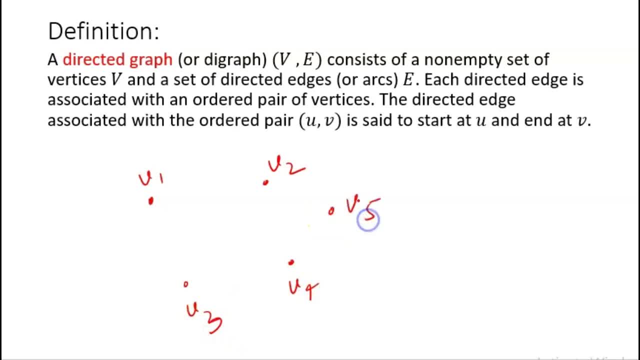 v3, v4 and v5. five vertices now i am joining the edges between them. so when i am joining the edges between them i am associating a direction, uh, with all the edges like: so here the edge is starting at v1 and going up to v2. here the edge is starting at v2, going up to v5. i can draw an edge between 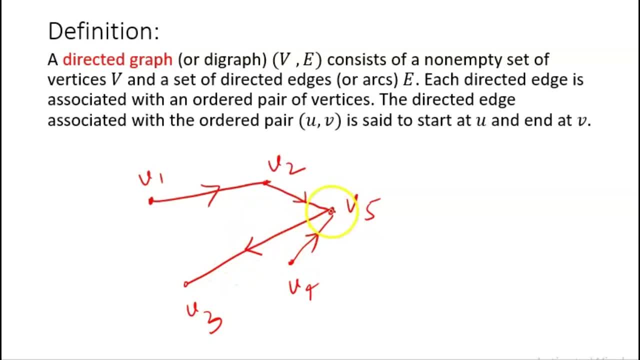 v3 and v5 and which is starting at v5 going up to v3. so in this graph, all the edges are having a direction which is associated with it. so this is an example of a directed graph. now, if i have to represent the edge, i will represent the edge by the ordered pair, like: 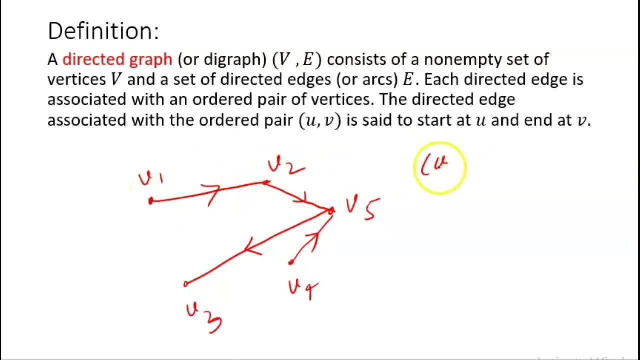 if i have to represent this edge which i have drawn between v1 and v2, so i will represent it by the ordered pair, ie v1 and v2. they have to be ordered so that there is an interface at V1 and V2. 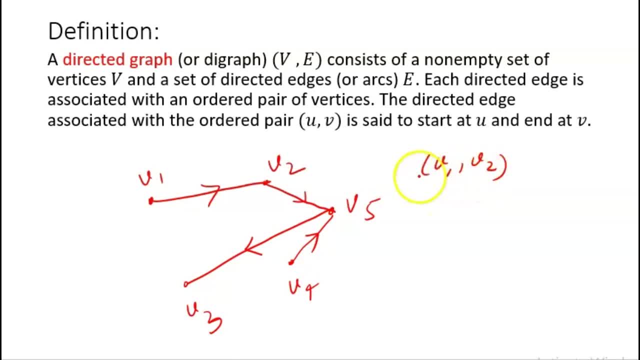 v1 comma v2 and i hope you understand v1 comma v2 is not equal to v2 comma v1, because when i am drawing the edge it is starting at v1. so v1 is the initial vertex and v2 is the terminal vertex. 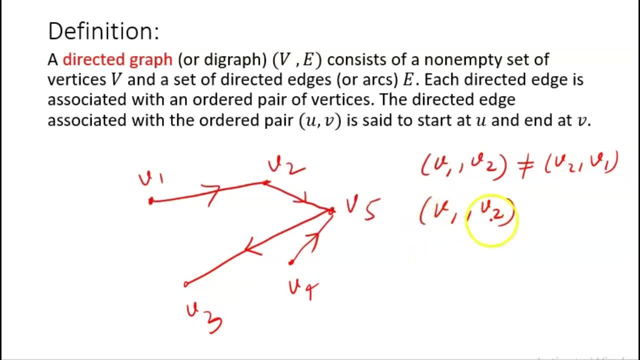 so in that order it should be written right, because this is an ordered graph, or rather this is a directed graph. pardon me for the use of the word ordered, because we are using the term directed graph. so this is a directed graph, so for each edge we have, you know, a sense of direction. 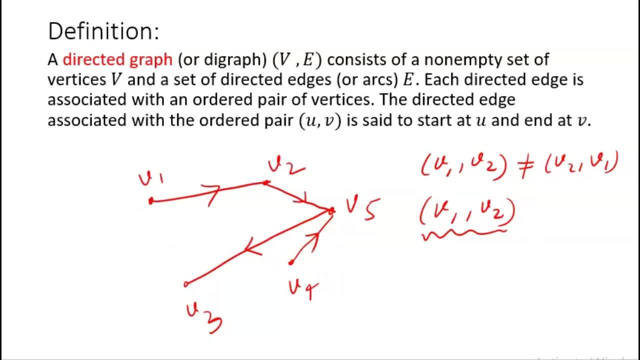 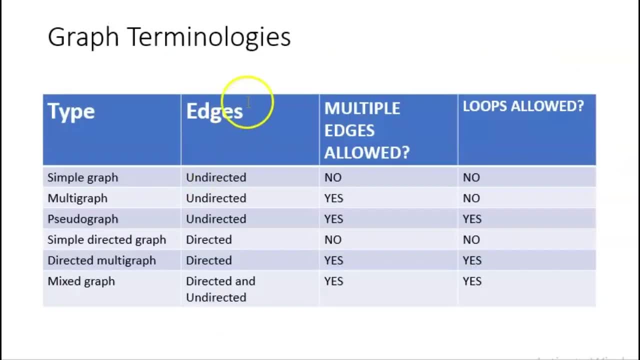 associated with it. now we have seen two things: one is undirected graph and another is, uh, directed graph. now there are different terms which we use, so let us look at them one by one. so the first thing that we are going to talk about edge simple graph. so you see what is the- you know- property of simple graph that edges will be. 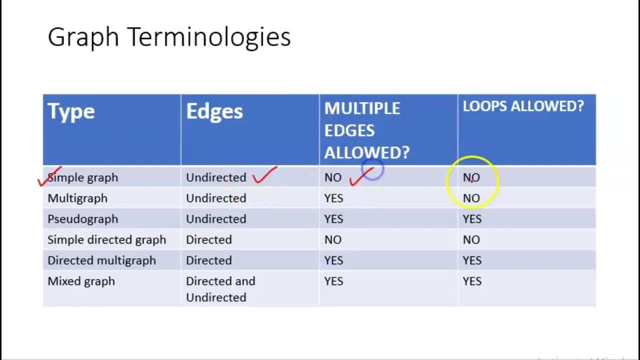 undirected, the multiple edges will be allowed and the loops will be allowed. but before i talk about this, be clear about what do you mean by multiple edges and loops. so suppose i take two vertices, v1 and v2, and if i join more than one edge between them, then we say that there are multiple. 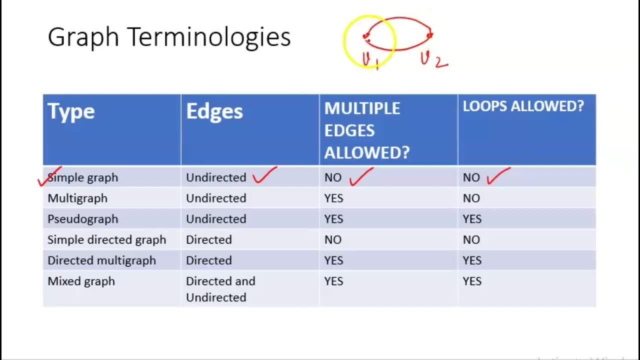 edges between two vertices. right it may. it may be three edges also, it may be any number of edges. the idea is that the number of edges should be more than one. and when i talk about loop, so suppose i take a you know three vertices- v1, v2 and v3- and suppose i join it like this: uh, there is an edge between v1 and v2. there is an. 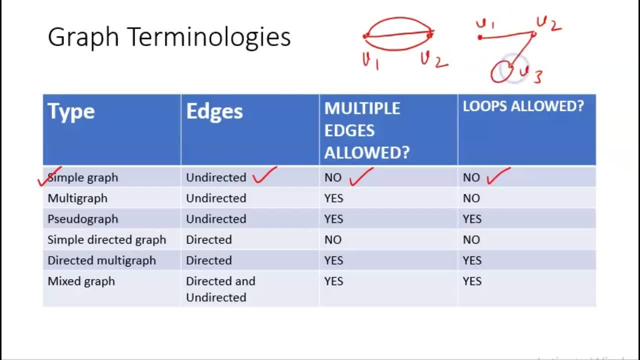 edge between v2 and v3 and suppose i join an edge between v3 and v3. so here this, this edge which, which is associated with just one vertex, is known as loop right. so in this graph i have just two vertex and between them there are three edges. so these are, this is a you know. these are three. 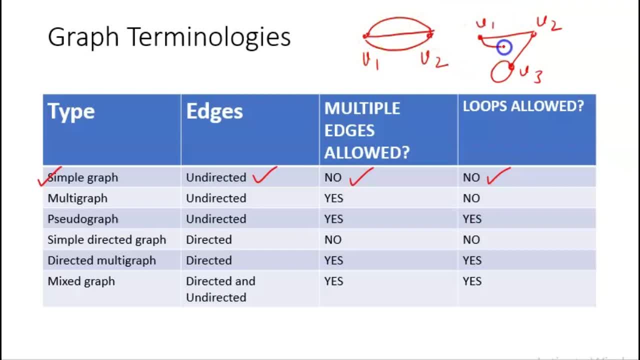 multiple edges between these two vertices. now, uh, in this graph we have both the multiple edges as well as the loops. so when we talk about the simple graph, simple graphs are those graphs in which the edges are undirected and multiple edges and loops are not present. so, for example, 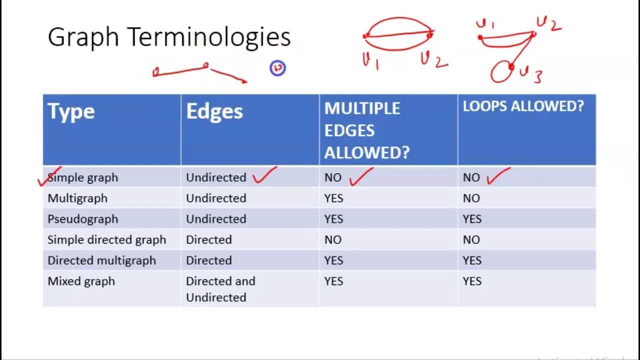 if i draw just one simple graph here here i have four vertices: v1, v2, v3 and v4, and between- uh, this there are, i mean between any two vertex, we have just one edge, right, there is no multiple edge, and similarly there is no loop here. so this is an example of a simple graph. 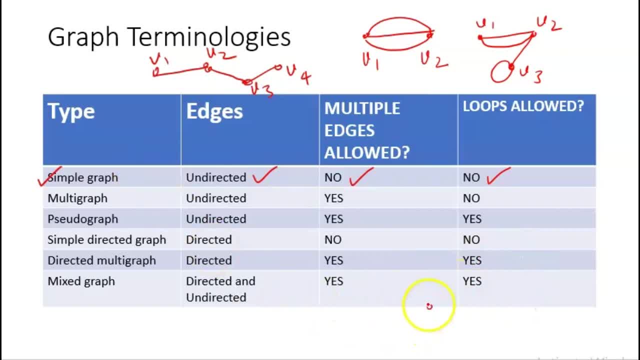 if i ask you draw a multi-graph, so let me draw a multi-graph. i have taken four vertices and i am joining them like this and suppose i join this and this. now, between these two vertices we have more than one edge. so this is an example of a multi-graph, because in multi-graph we have 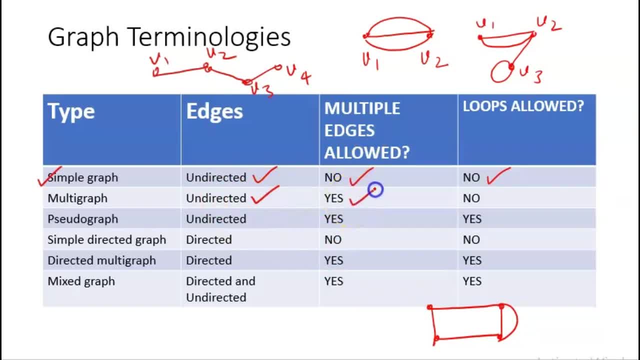 undirected edges, the multiple edges are allowed, but loops are not allowed. when we have a situation where the edges are undirected and multiple edges are also present and loops are also present, so those graphs are known as pseudographs. so for example, suppose i draw a pseudograph. 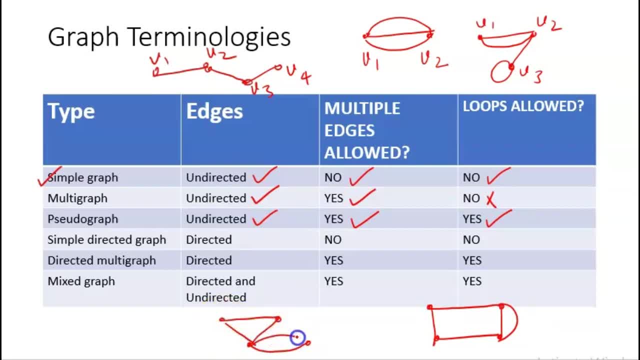 here. so between two vertices we have, uh, you know, multiple edges and with this vertex we have a loop, right? so this is an example of a pseudograph, because here the multiple edges are also present and loops are also present. okay, so we have three terms that we are using simple graph. 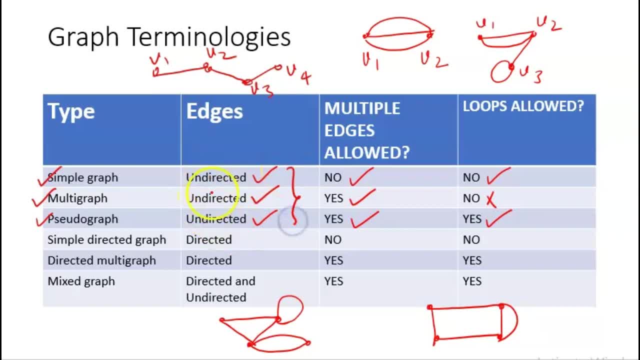 multi-graph and pseudograph. in this the edges are undirected and i hope you have understood that if we have a simple graph, we have a loop right. so this is an example of a pseudograph. the multiple edges are not present, loops are also not present. then that is simple graph. 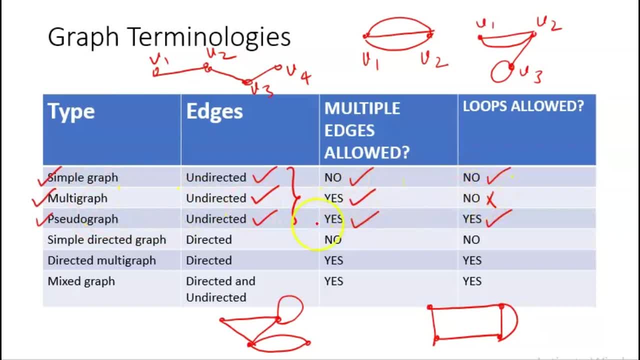 multi-graph when the multiple edges are present but loops are not present. pseudograph when the multiple edges and loops both are present. similarly, when we talk about directed graph, we have two terms. one is simple directed graph and another is directed multi-graph. here we are not, you know, using the term pseudo term. right, this is just terminology, so don't be fussy about that. 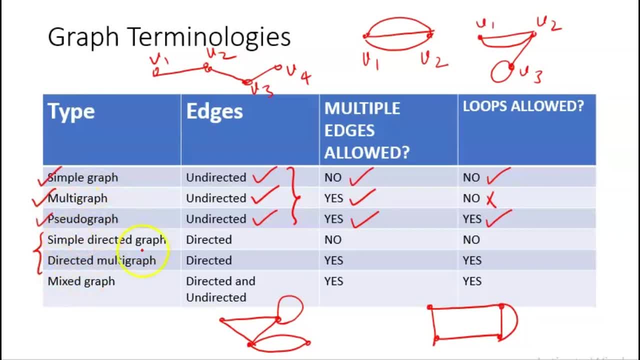 why we are not using pseudo multi-graph, because it is just the terminology that we have already, you know, accepted. so suppose i uh draw one example of simple directed graph. so this is a simple directed graph between: uh, you know, there is no multiple edge, the edges are directed, but there is 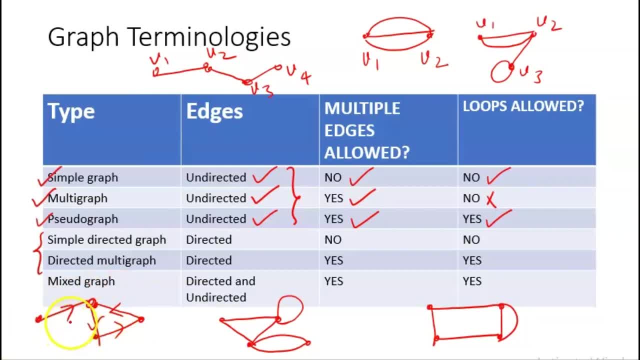 no multiple edge present between any two uh vertex and similarly there is no loop present between no2. similarly, if i draw a directed multi-graph, how uh it will look like? so let me draw a directed multi-graph. so here suppose i draw multiple edges between these two vertices and suppose 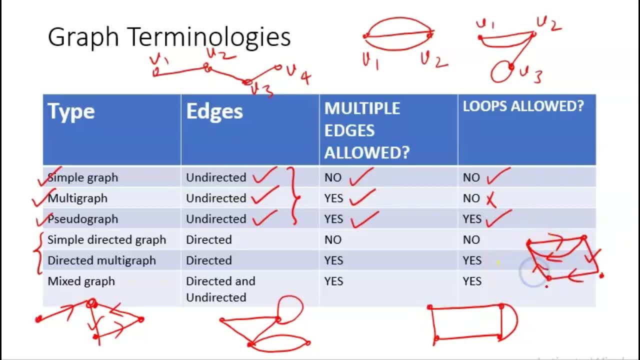 i draw edges like this right, and on this vertex, suppose i draw a loop as well. so this is the example of a directed multi-graph. finally, we have something known as mixed graph. so in mixed graph we have, uh, you know, both kind of edges, directed as well as undirected. so let us 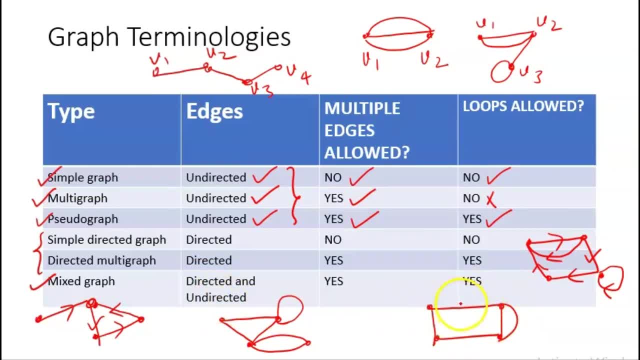 take this example, and here let us let me draw it further. so suppose i draw this edge which becomes a directed edge, i draw this edge which also becomes a directed edge, but there is no direction. i am associating with this edge, with this edge and this edge, and let me draw a- uh, you know, multiple. 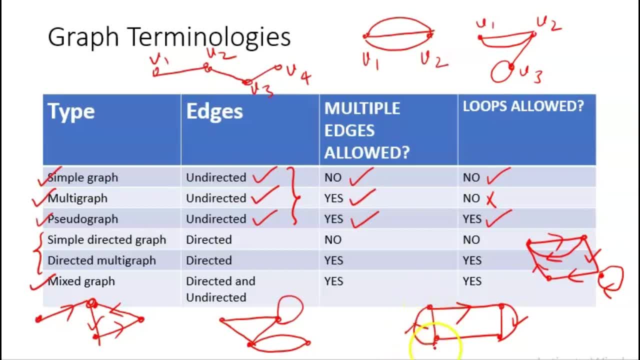 edge between these two. one is directed, another is undirected, and let me draw a loop also over this. now, this is an example of a mixed graph. why it is an example of mixed graph? because it has multiple edges and because between these two vertex we have more than 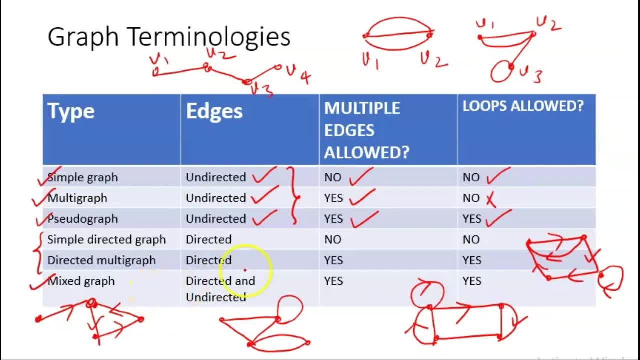 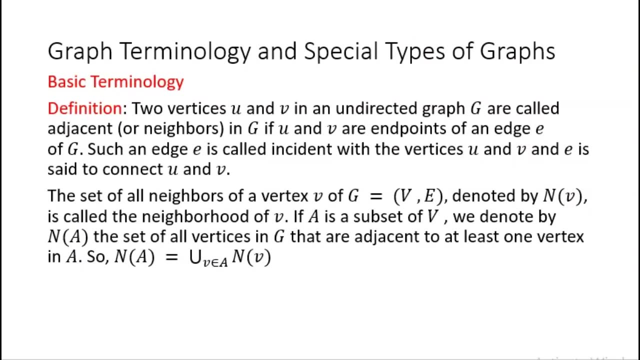 one edge between these two vertex. we have more than one edge. it has both kind of edges, directed as well as undirected. so this is an undirected edge, this is a directed edge. so, uh, this kind of graph is known as mixed graph. okay, okay, so, uh, now let us look at some more terms, and the first term that we are going to look at is: 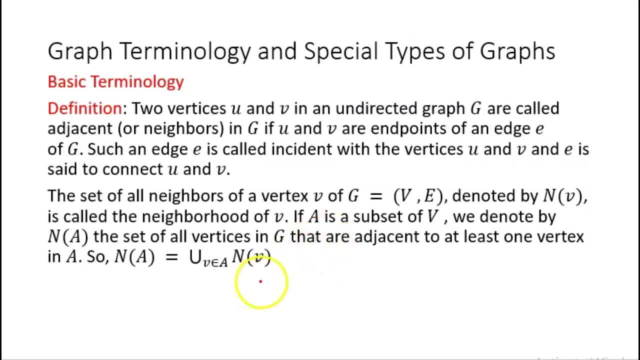 adjacent vertex. of any given vertex, you can read the definition and pause the video. if you want to create your own notes, you can write the definitions as well. i am going to explain this through an. so let me first write or draw a simple graph right which has four uh vertices: a, b, c, d. let me draw one. 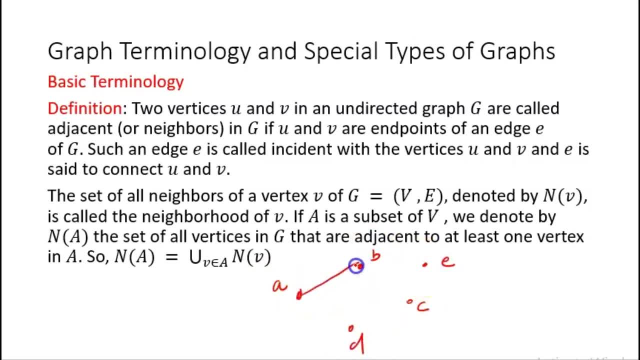 more vertex e now, if i uh draw different edges between them. so let me draw these edges right now. first thing, i ask you that if i look at the vertex a here, this vertex a is uh associated or joined to just one vertex b, so a and b are said to be the adjacent vertices. if i ask you what is the? 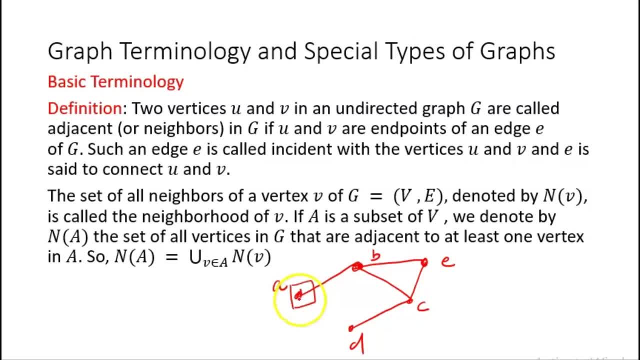 adjacent adjacent vertex of a. so the adjacent vertex of a is just one vertex, that is, b. next, if i ask you, what are the adjacent vertices of b? so adjacent vertices of b are: a because there is an edge between b and a. e because there is an edge between b and e. 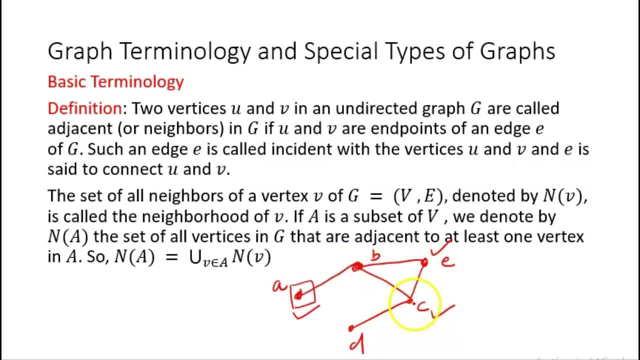 and c, because there is an h between b and c right. similarly, what are the adjacent vertices of c? the adjacent vertices of c are b, e and d. what are the adjacent vertices of d? it has just one adjacent vertex, that is c. and finally, if i ask a vertical vector, 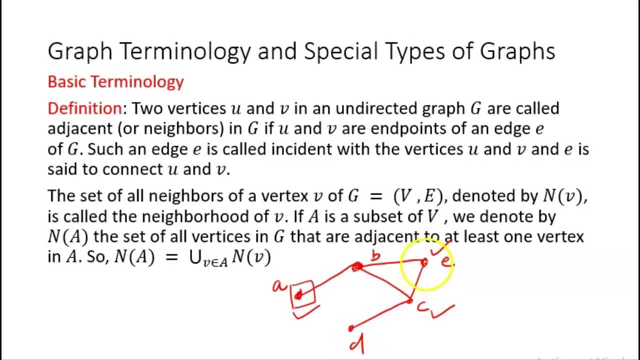 you what are the adjacent vertices of the vertex e? so there are two adjacent vertices, that is, b and c. so i hope you got about what do i mean by adjacent vertices. similarly, the another term that they define is the neighborhood of a vertex. so, for example, if i ask you that, what is the? 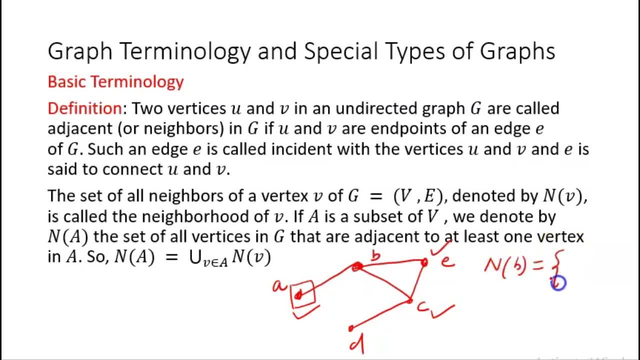 neighborhood of the vertex b. so it is the set of all those vertices which are adjacent to the vertex b. so it will have a, it will have e and it will have c, because those vertices which are adjacent to b are a, e and c. if i ask you, what is the neighborhood of the vertex d? so the neighborhood. 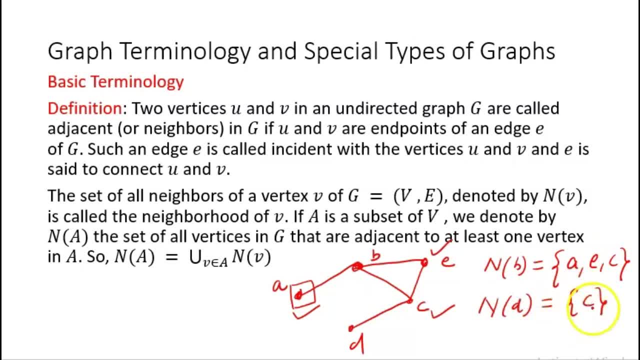 of the vertex d just contain one vertex, that is, the vertex c, right? if i ask you what is the neighborhood of the subset like, let me take a subset a of the vertices. so suppose i take the subset a and c, and if i ask you what is the neighborhood of a, so it will be. 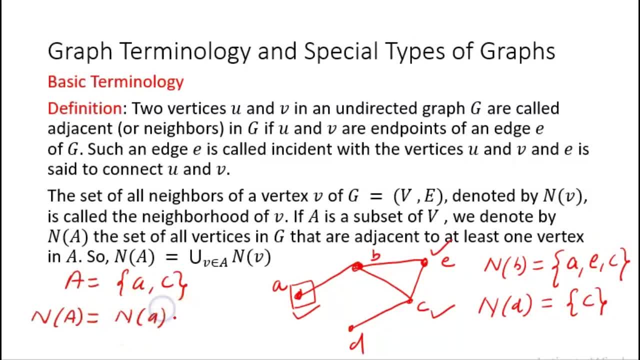 the neighborhood of the vertex a union, the neighborhood of the vertex c, and this is what the definition is: that if i have a subset a of the set of vertices v, then the neighborhood of the subset a is the union of the neighbor, neighbors of all the vertices which. 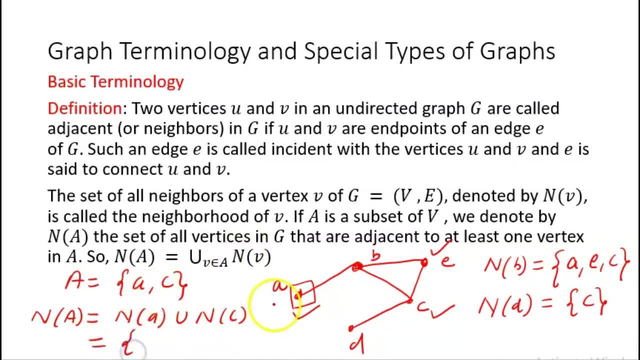 belong to the set a. so in this case, what is the neighborhood of a? neighborhood of a is b and union. what is the neighborhood of c? neighborhood of c is b, e and d. so i have b, e and d. so if i take the union i will get b, e and d. so this is the concept of neighbors and neighborhood, now one. 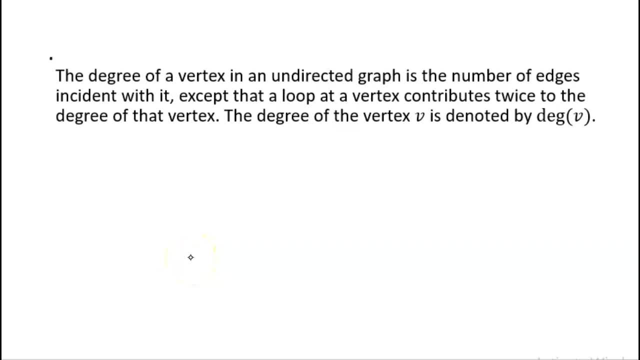 more term that i want to define is known as a degree of a vertex. so the degree of a vertex in an undirected graph is the number of edges incident with it, except that a loop at a vertex contributes twice to the degree of that vertex. the degree of a vertex, v, is denoted by v. let us understand it through this example. 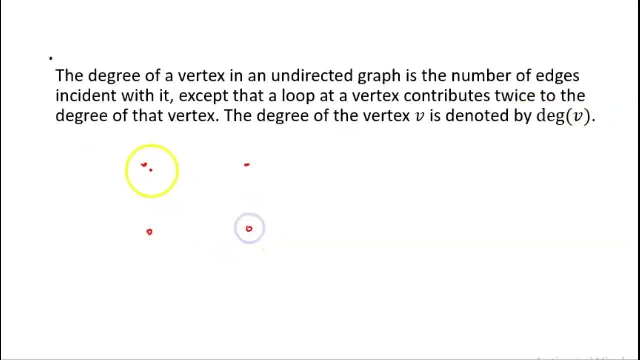 so suppose i have a graph here, And in this graph I have, suppose, five vertices: A, B, C, D and E, And let me join these edges between them right. Let me write one more, vertex F. 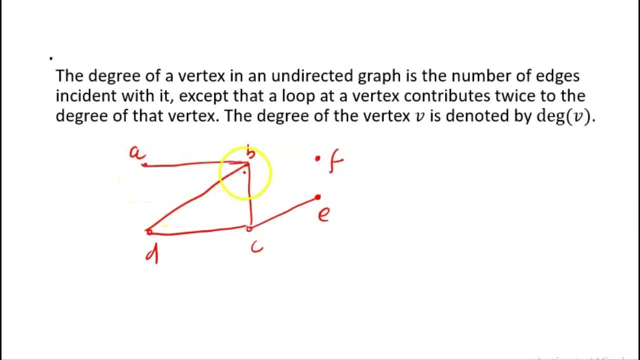 That will be important because it will help you to understand other terms as well. Now, if I ask you what is the degree of A? So if I ask you what is the degree of the vertex A? Degree of the vertex A is one, because there is just one edge, which is incident at the vertex A. right, 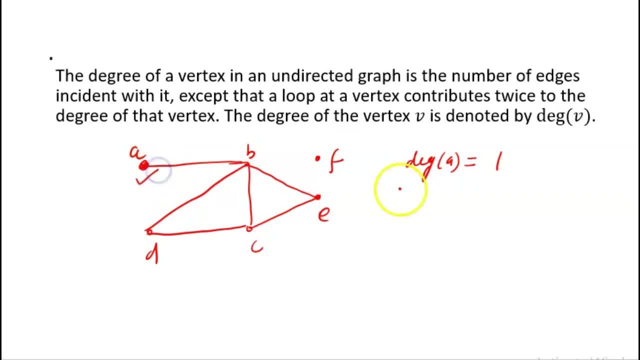 This is just one edge which is incident at the vertex A. If I ask you, what is the degree of the vertex B? So the degree of the vertex B, how many edges are incident at B? One, two, three, four? 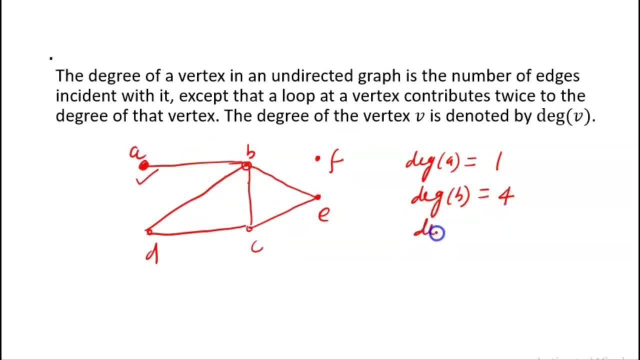 So the degree of the vertex B. If I ask you, what is the degree of the vertex C? So how many edges are incident at C? One, two, three. So the degree of the vertex is three. What is the degree of the vertex D? 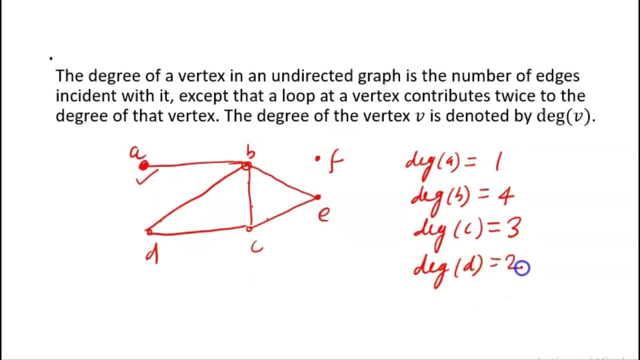 So how many edges are there? One and two, So it is equal to two. If I ask you what is the degree of the vertex E, So that is also two. And if I ask you what is the degree of the vertex F, 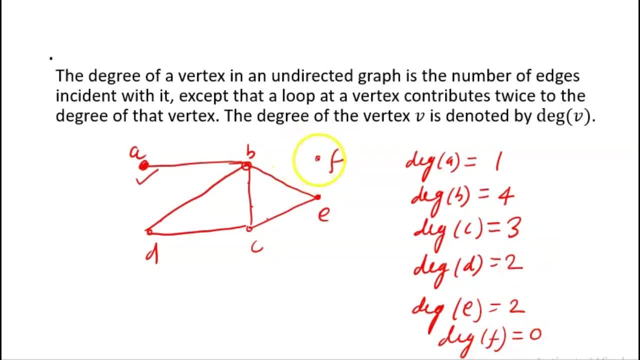 So it is equal to zero, because there is no edge incident at F. So I hope you have understood the meaning of the degree of a vertex. If the degree of a vertex is one, then it is known as a pendant vertex right. 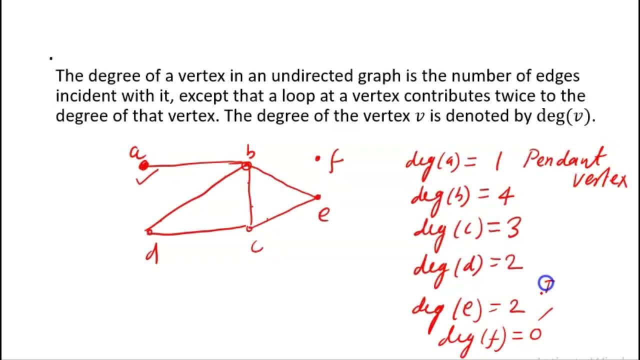 And if the degree of a vertex is zero, that vertex is known as isolated vertex, Yes or no? So this term- sometimes they use the pendant vertex- means its degree. If the degree is one, isolated vertex means its degree is zero. 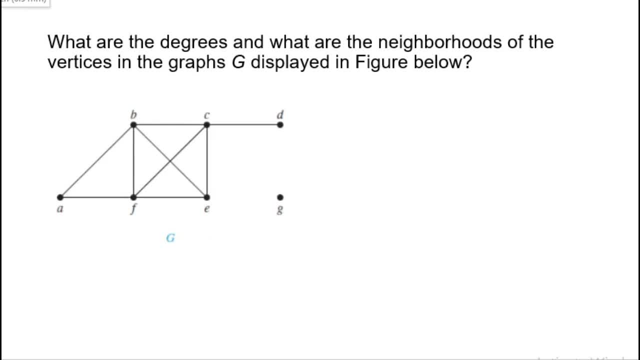 Now, just to be clear about the terms that we have just understood. let us quickly solve this problem. So what are the degrees and what are the neighborhoods of the vertices in the graph G displayed in the figure below right? So let us answer this question. 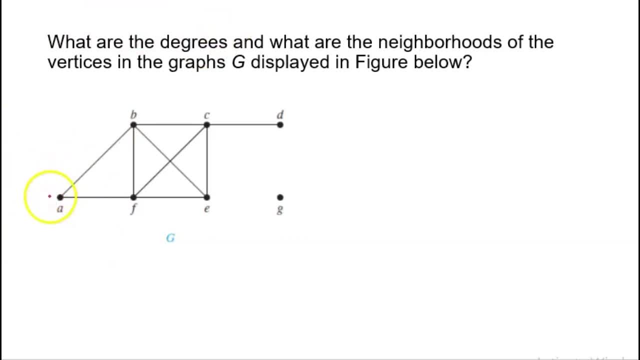 And I am going to write the: what is the degree of the vertices over it? So what is the degree of A? So the degree of A is two right Because degree of there are two edges which are incident at A. 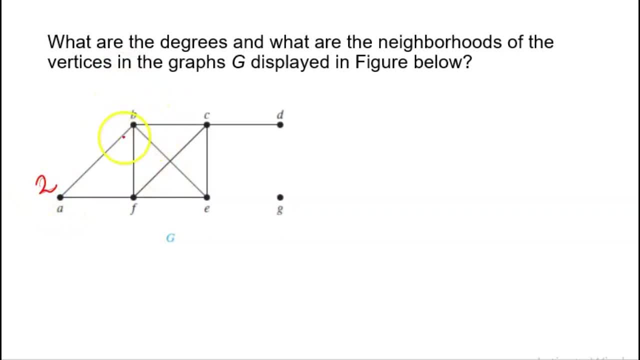 So the degree of the vertex A is two. What is the degree of the vertex B? One, two, three, four. So there are four edges incident. So the degree of the vertex B is four. What is the degree of the vertex C? 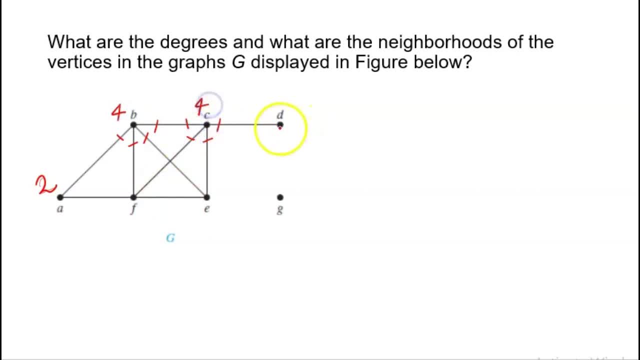 One, two, three, four, So four. What is the degree of the vertex D: One. What is the degree of the vertex E? One, two, three, So three. What is the degree of the vertex F? 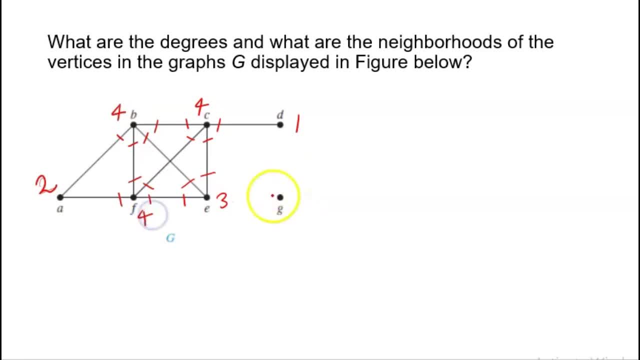 One, two, three, four, So four. And what is the degree of the vertex G? That is zero. So these are the degrees of the different vertices. Now, if I ask you that, what are the neighborhoods of the vertices in the graph A? 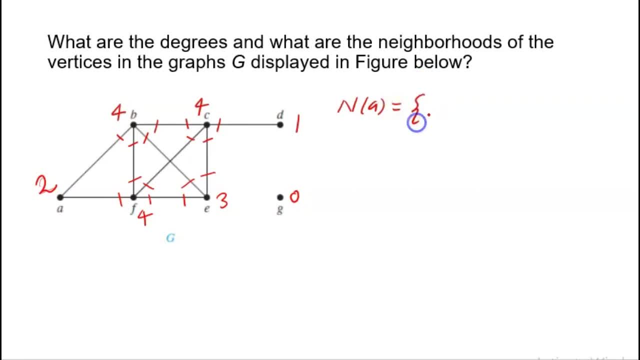 So if I ask you, what is the neighborhood of A? So the neighborhood of A are the vertices, the set which contains the vertices B and F. If I ask you, what is the neighborhood of B? So the neighborhood of B will contain A, C, E and F. 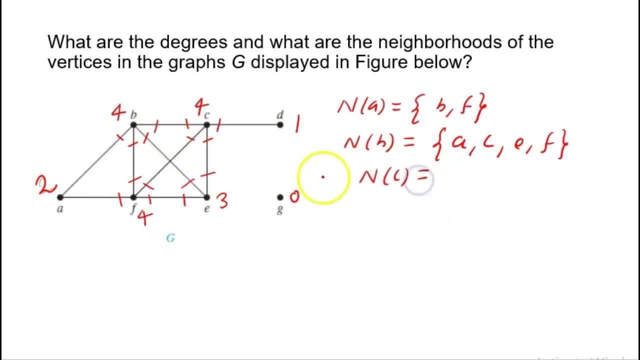 The neighborhood of C will be the vertices B, D, E and F. The neighborhood of the vertex D will be just the vertex C. The neighborhood of the vertex E will have three, you know, vertices: F, B and C. 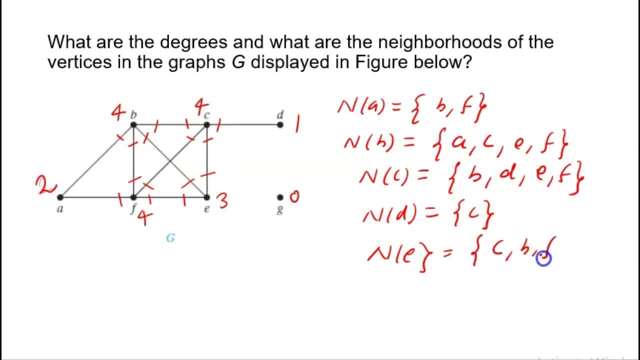 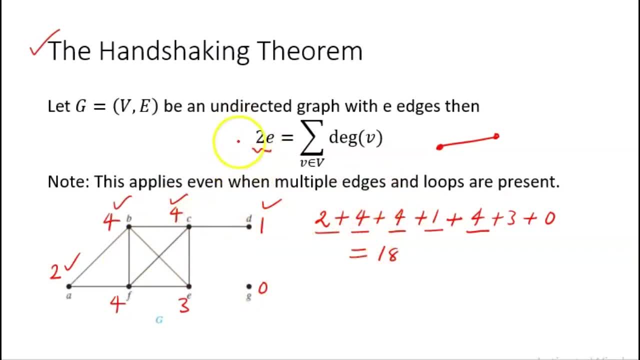 And the neighborhood of the vertex G is: let me draw this like this: A, B, C and E. And the neighborhood of the vertex G is: let me draw this like this: A, B, C and E, And, as per the hand-stacking theorem, how many edges it should have. 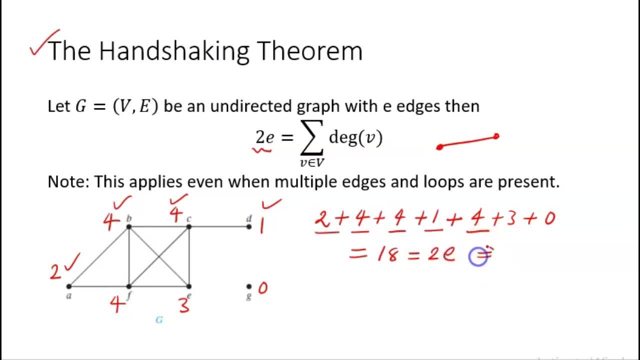 So this would be equal to twice the number of edges, means the number of edges should be equal to 9.. So let us count the number of edges. So this is the first edge, second, third, fourth, fifth, sixth, seventh, eighth and 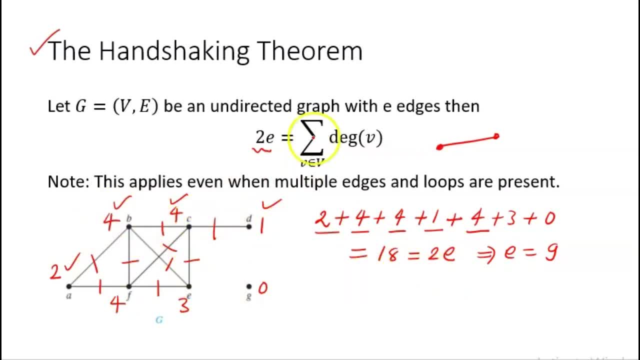 ninth. So we can clearly see that it has 9 edges and that we can also see from the hand-stacking theorem. So one thing that I hope you have already understood: that the number of edges, if you multiply it by 2, it will give you the sum of the degree of the vertices present in the 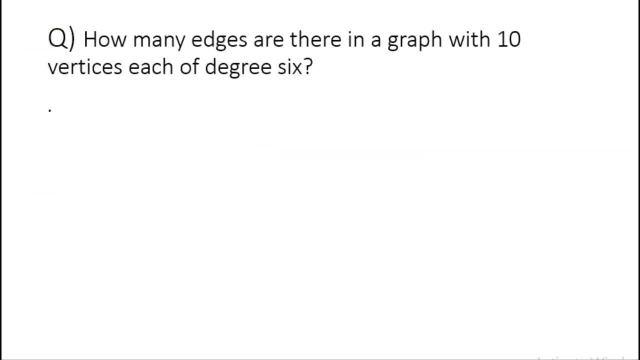 graph Right To understand this. let us quickly solve this problem. How many edges are there in a graph with 10 vertices, each of degree 6?? So how will I solve it? How many vertices are there? The number of vertices is equal to 10, and each of the vertices vertex is of degree. 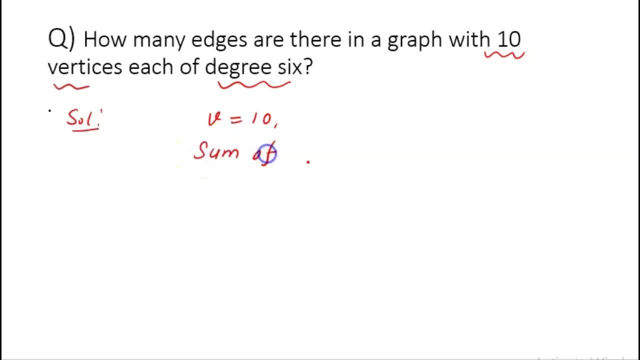 6.. So what is the sum of degrees of the vertices? It is equal to 6 into 10, because each vertex is of degree 6, and there are 10 vertices. So the sum of degrees 6 into 10 is equal to 60.. 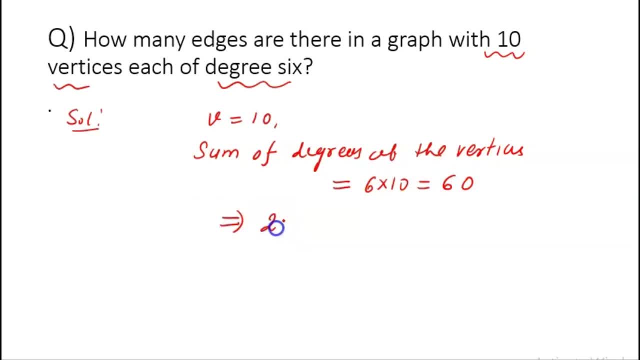 Right. So we know from the hand-stacking theorem that twice the number of edges should be equal to the sum of the degree of vertices, that is 60. So it means that E should be equal to 30. So how many edges should be there in the graph? 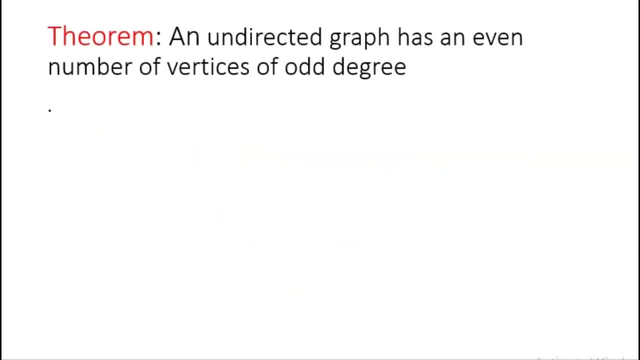 There must be 30 edges. There is a very important result associated with, or that is a kind of corollary to, the hand-stacking theorem, that in an undirected graph has an even number of vertices. Let me repeat this. 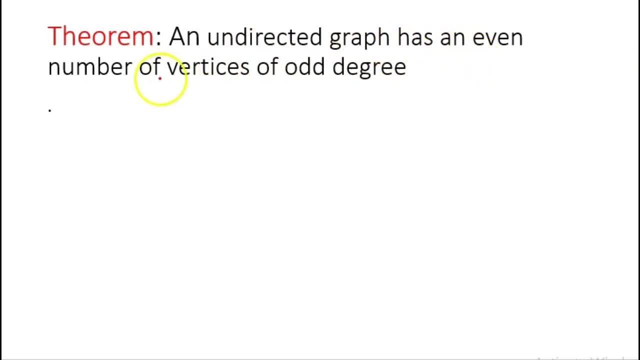 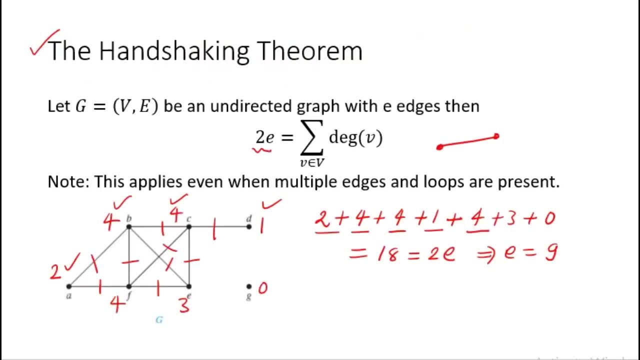 An undirected graph will always have an even number of vertices of odd degree. So to understand this, let us go to the previous example And if I look at this example here, how many vertices are there of odd degree? So this vertex is of even degree. this vertex is of even degree, even degree. 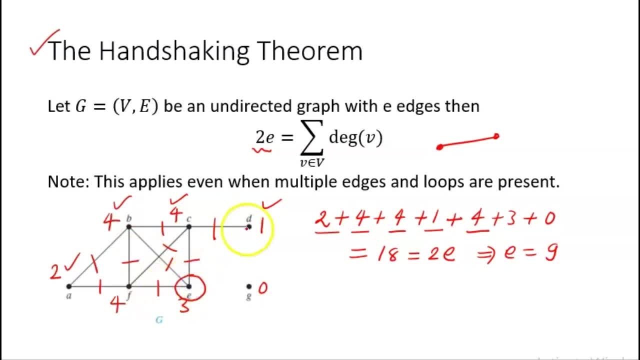 The vertex E here is of odd degree. So this vertex is of even degree. this vertex is of even degree, even degree. The vertex E here is of odd degree and the vertex D here is of odd degree. So the number of vertices of odd degree are two, which is even. 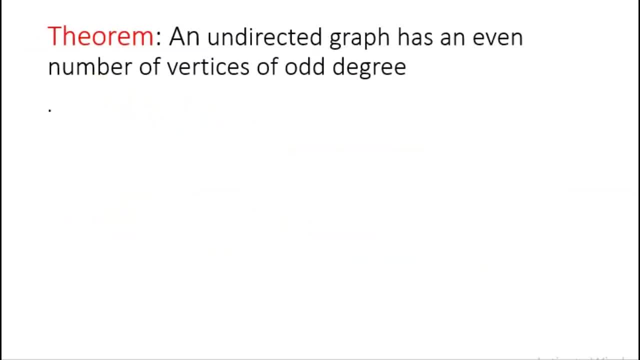 I hope you got it. If you draw any graph, let me draw one random graph. suppose I draw a graph like this, any random graph. I am not thinking, I am just randomly drawing it. Let me draw one more vertex, right? 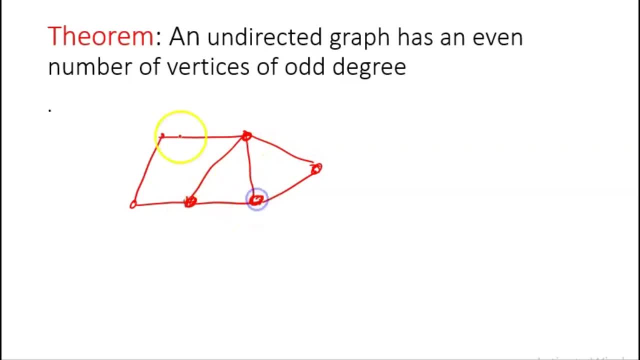 So suppose I have this graph And if I count the number of vertices, so what is the degree of this: 2, degree of this, 2, degree of this, 3, degree of this, 4, degree of this, 3, and degree of? 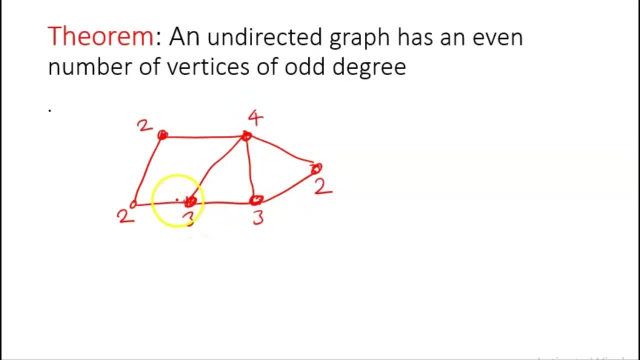 this: 2.. So how many vertices are there of odd degree? There are two vertices of odd degree, which is actually even in number. There is a very simple proof of this result And I would like all of you, if you are watching this video, please try to write a proof of. 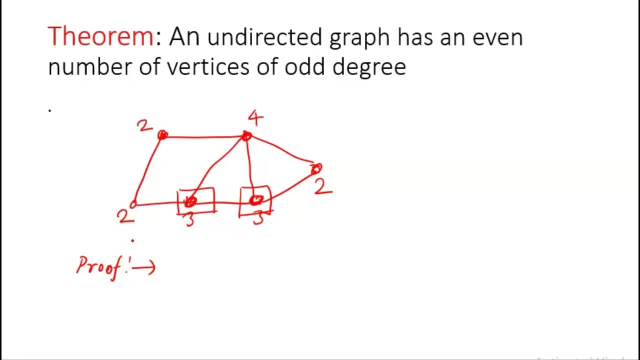 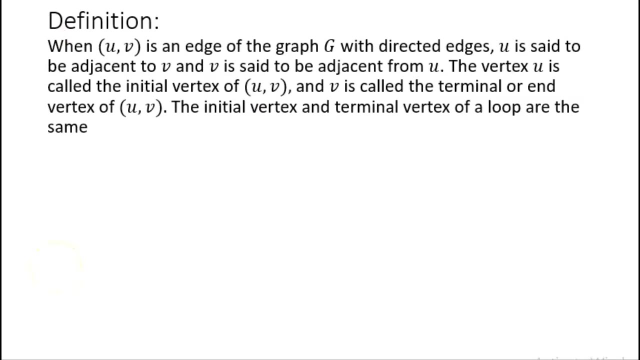 this result And put the proof in the comment section of it. It is very simple: You just have to use the basic logic of Hand-Sacking Theorem and you will be able to prove this. Now let us look at the things related to under sorry directed graph. 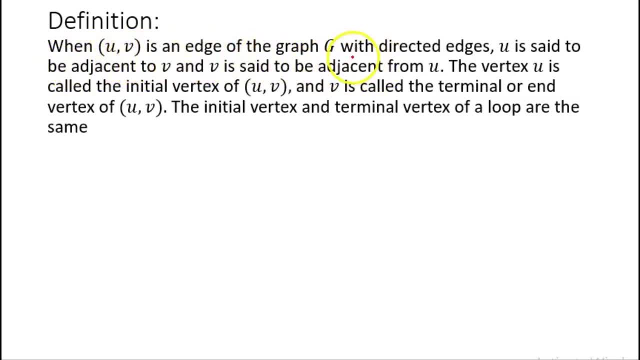 So let u comma. v is an edge of a graph G with directed edges. u is said to be adjacent to v And v is said to be adjacent from u. These are just the play of words. The vertex u is called the initial vertex of uv and v is called the terminal vertex. 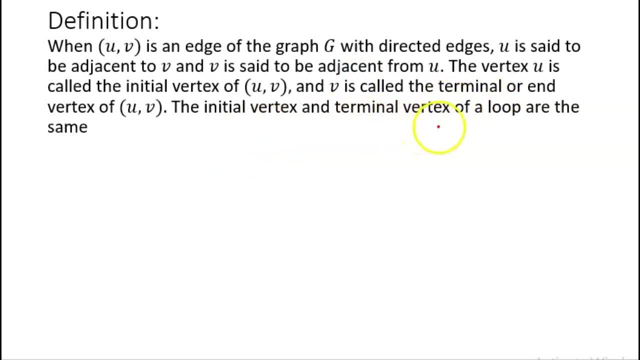 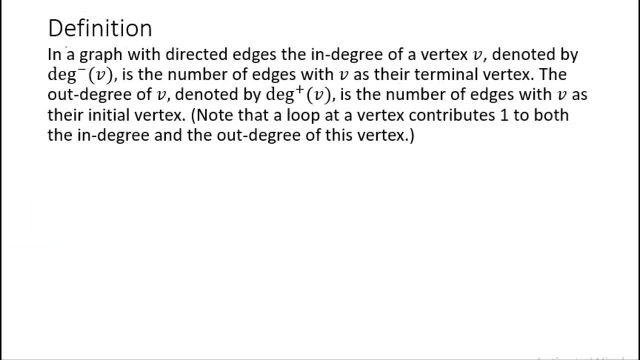 or end vertex of uv. The initial vertex and terminal vertex of a loop are the same. I think it is nothing special here. You already have seen that thing in our discussion- But this is important. In a graph with directed edges. There are two terms that we are going to define. 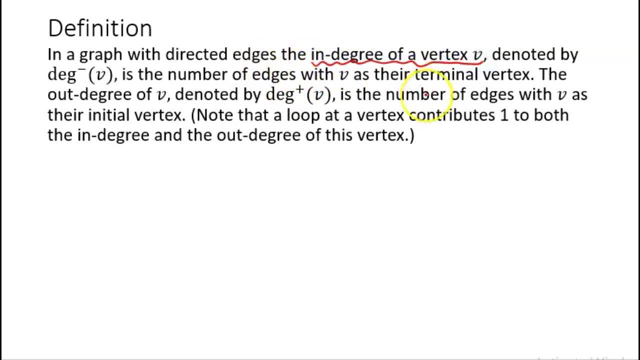 One is known as in-degree of a vertex and another is known as out-degree of a vertex v. So let us look at the definition In a graph with directed edges: the in-degree of a vertex v denoted by degree minus v. 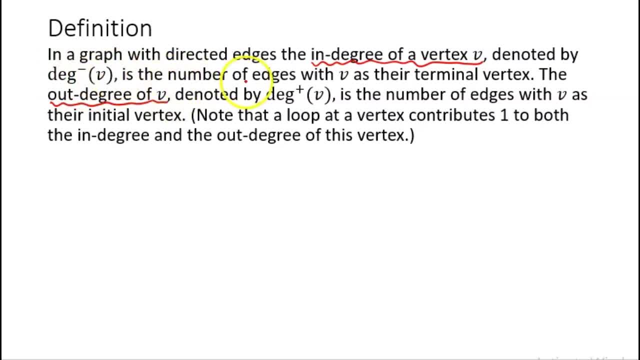 This is the representation of: in-degree- is the number of edges with v as their terminal vertex. In-degree means that the number of edges which are having v as their terminal vertex And the out-degree denoted by degree plus v, is the number of edges with v as their initial. 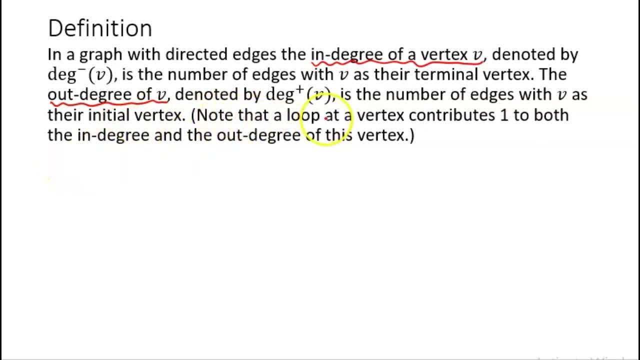 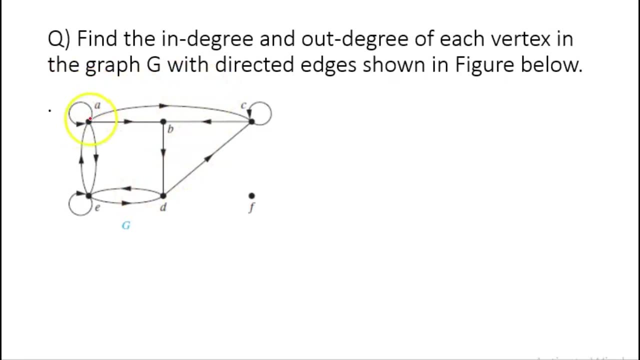 vertex. Note here that a loop at a vertex contributes one to both the in-degree and the out-degree of that vertex. To understand this, let us look at this example. Let us look at this example. So if you have this graph A and if I ask you that, what is the in-degree of the vertex? 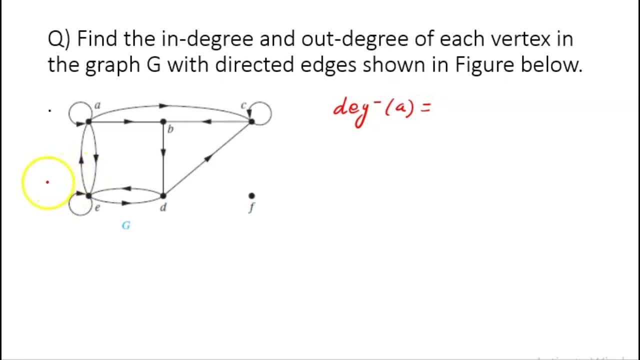 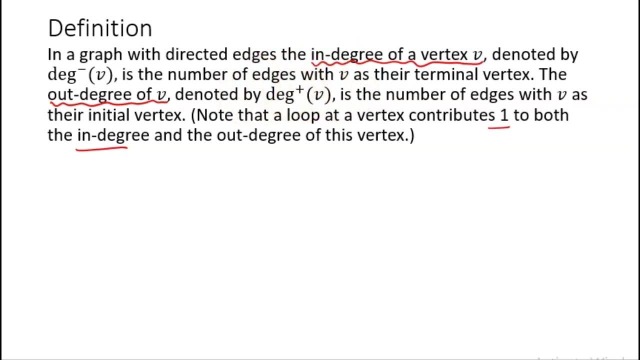 A. So what is the definition? The in-degree of a vertex is the number of edges, which are you know. look at the definition again In a graph with directed edges. in-degree of a vertex is the number of edges with v as their terminal vertex. 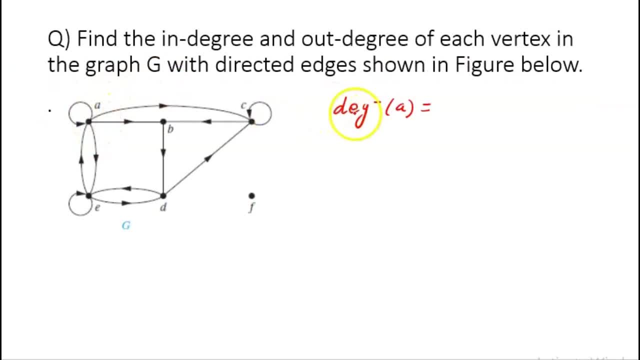 It means what? That we are going to define the in-degree of A by looking at how many edges are entering into A. Okay, So the number of edges which are entering into A. so you can see that this edge, this edge is entering into A because A is the terminal vertex. 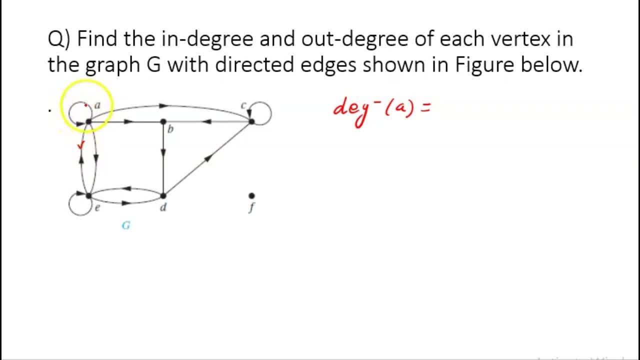 And there is a loop over here. So this will also contribute that One to the in-degree. So in-degree of A is two, because two edges are entering into this. This is one edge and another is the loop. If I ask you, what is the in-degree of the vertex B? so how many edges are entering into? 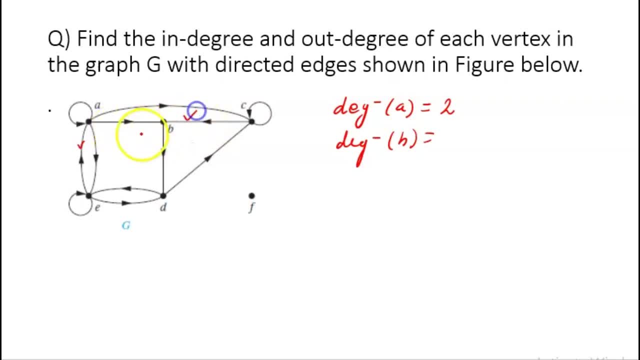 it. So one and then two. This one is also entering into B and this one is also entering into B. So in-degree is of B is two Means for B. these two edges have their terminal vertex, So in-degree of B is two. 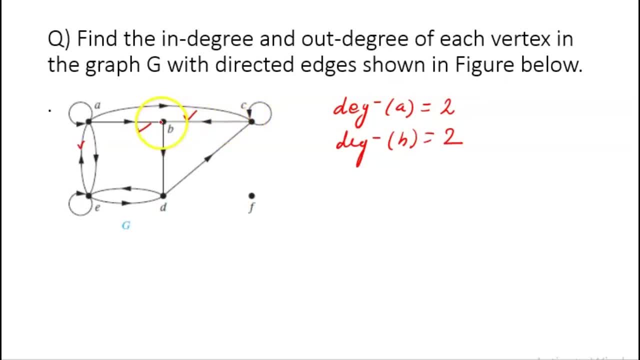 So in-degree of B is two, So in-degree of B is two, Which will have their terminal vertex HB. So just to understand it, You can just see that those you know number of edges, or those edges which are entering into it, are contributing to its in-degree. 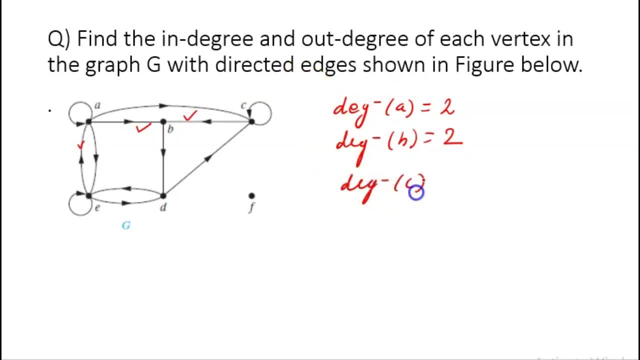 If I ask you what is the in-degree of the vertex C? so in-degree of the vertex C is here, This edge is entering into C, This edge is entering into C And the loop is also entering. So in-degree is three. 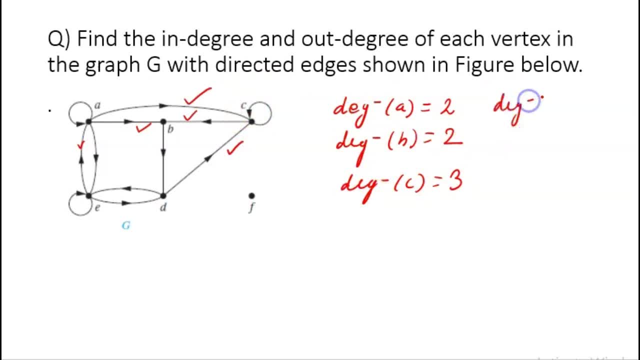 This is the loop. Now this edge is also entering into C. In-degree is three And loop The last edge. a loop already exists, end of every part. So end of every part. What is the in-degree of vertex D? 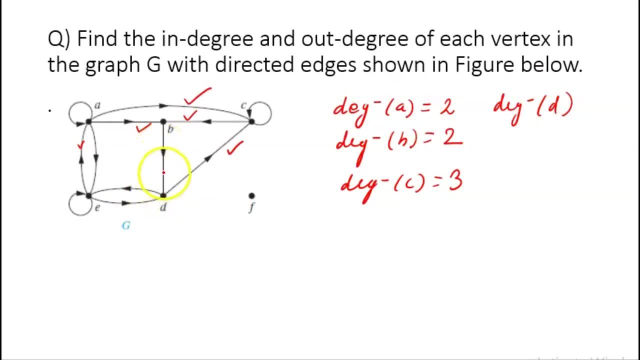 So in-degree of vertex D is B. this edge is entering, this edge is entering, so is equal to 2.. What is the in-degree of E? So how many edges are entering into it? This edge is entering, this edge is entering, and this loop is also entering, so it is equal to 3.. 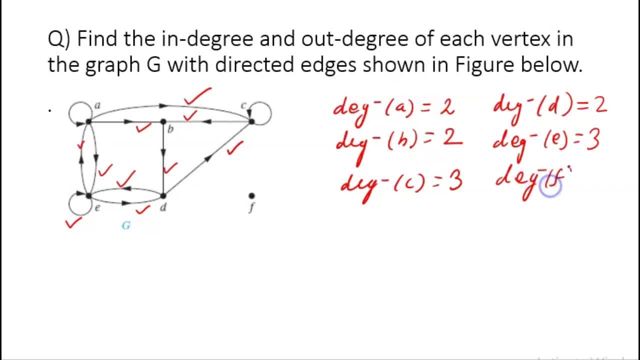 And what is the in-degree of the vertex F? So it is an isolated vertex. nothing is entering into it or nothing is leaving out, so actually is equal to 0.. I hope you got what is the meaning of in-degree of a vertex. 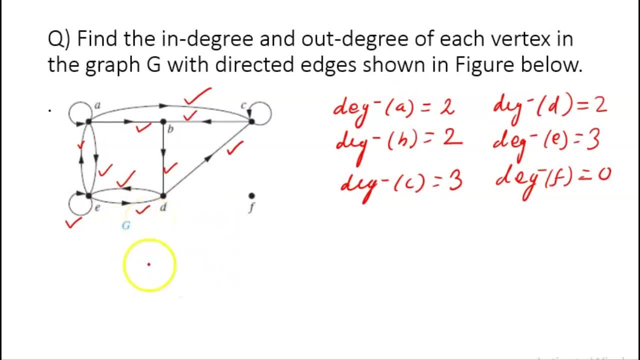 Now let us talk about the out-degree of each of them. So out-degree we represent by degree plus, so degree plus of A. So how many edges are coming out of A? So if you look at this, one loop, One loop is coming out of A, because loop contributes one to in-degree and one to out-degree. both 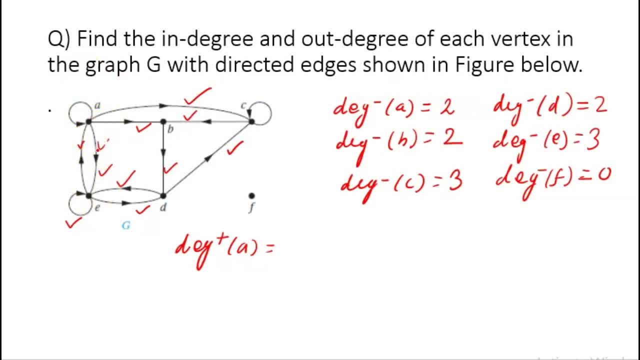 And this edge is also coming out. So the out-degree of A is this one: 1, 2, then this edge is also going out of A, and this edge is also going out of A. So 1,, 2,, 3, and 4.. 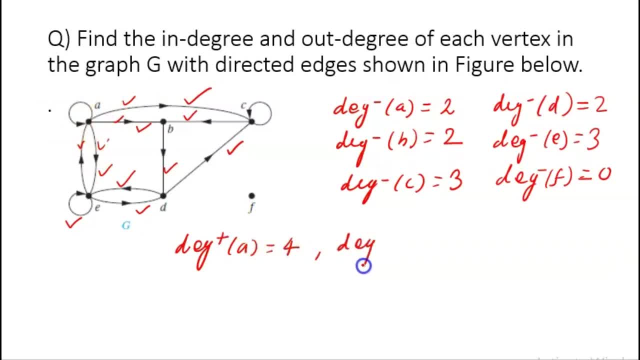 So out-degree of A is 4.. What is the out-degree of B? So from B, one edge is going out. So out-degree of B is equal to 1.. What is the out-degree of C? So from C this edge is going out. 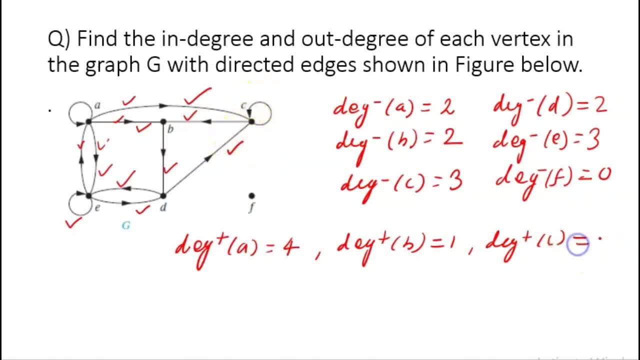 A loop is going out, So out-degree of C is also equal to 2.. What is the out-degree of the vertex D? So from vertex D, this edge is going out. this edge is going out, So 1 and 2.. 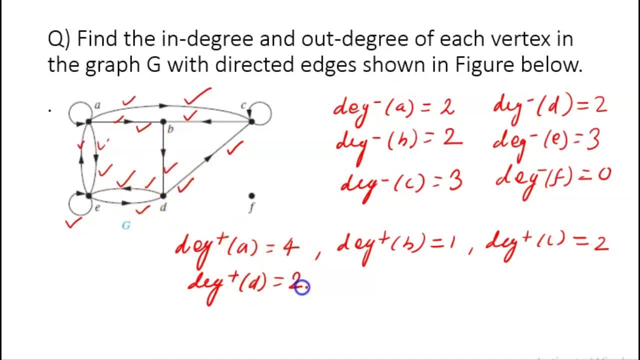 So 2 are actually coming and 2 are going, So it is equal to 2.. What is the out-degree of A? So 1 is the out-degree of the vertex E. so one edge, this edge is going out, this edge is going out and a loop is going out, so that is equal to 3.. 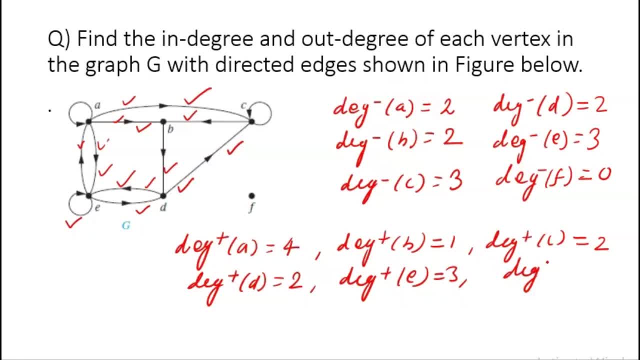 And what is the out-degree of the vertex F? So out-degree of the vertex F is equal to 0, because nothing is coming in or nothing is going out of the vertex F. So I hope you are clear about the in-degree and out-degree concept of a directed graph. 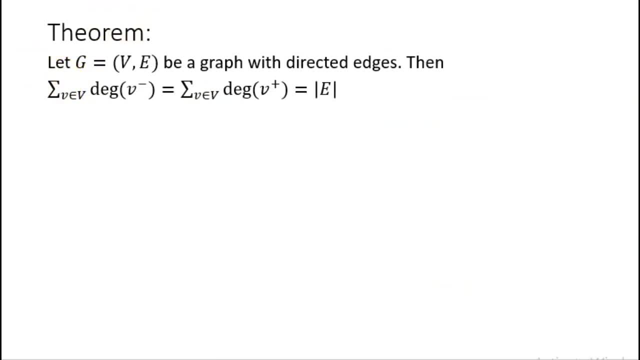 So the next thing is a theorem associated with the directed graph, And the theorem tells us that if G is equal to V, E be a directed graph, then the sum of in-degrees is equal to the sum of out-degrees of the vertices. 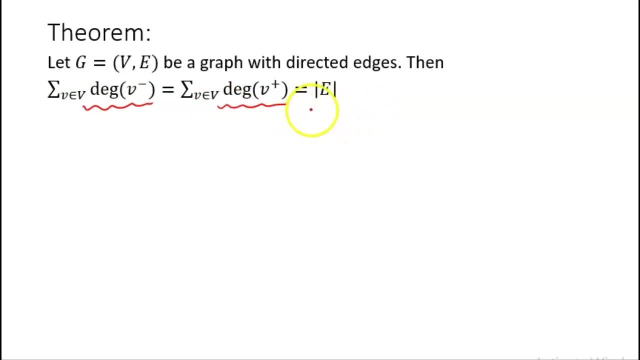 And that is equal to the number of edges present in the vertex. And that is equal to the number of edges present in the vertex. I hope you got it. If you didn't, let us go and see the previous example. If I look at this and let me change the color so that you don't get confused. 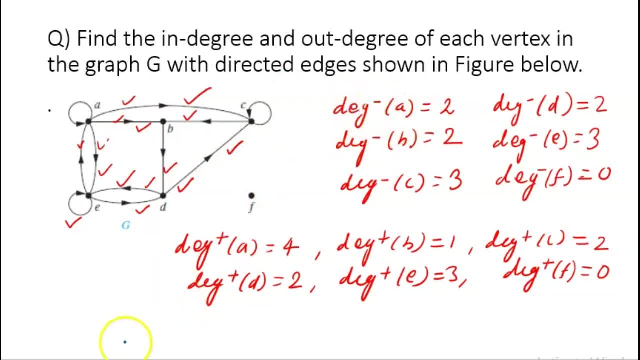 If I look at the sum of all the in-degrees. so here the sum of in-degrees is 2, because the in-degree of A is 2.. Then 2 plus 2,, 4,, 4 plus 3, how much? 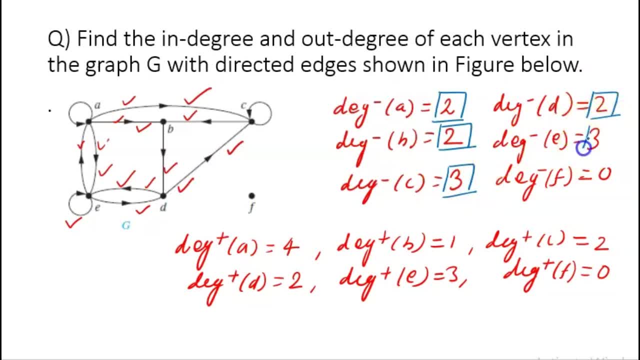 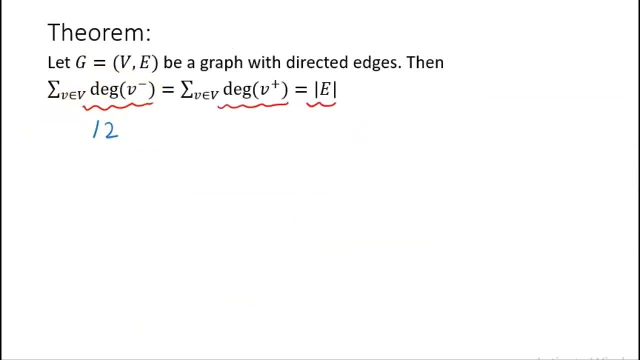 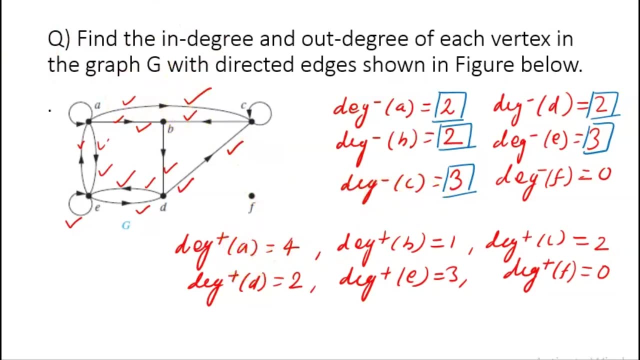 7,, 7 plus 2, 9,, 9 plus 3 is equal to 12.. So this term that we are getting here is equal to 12.. Now, if you look at the sum of out-degrees, so sum of out-degrees will be what? 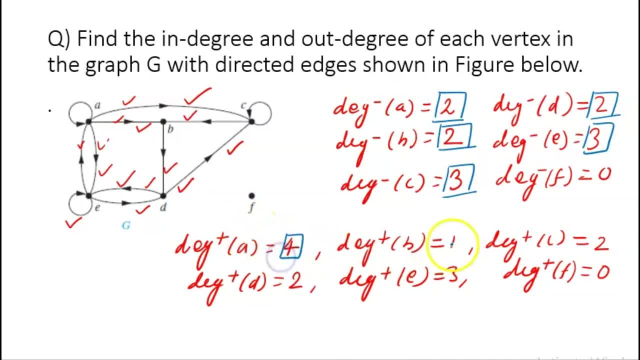 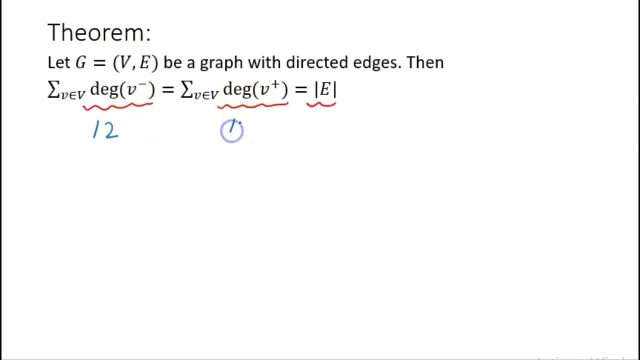 The sum of out-degrees will be 4 plus 1,, 5 plus 2,, 7 plus 2,, 9 plus 3,, 12 and plus 12.. So the sum of out-degrees is also equal to 12.. 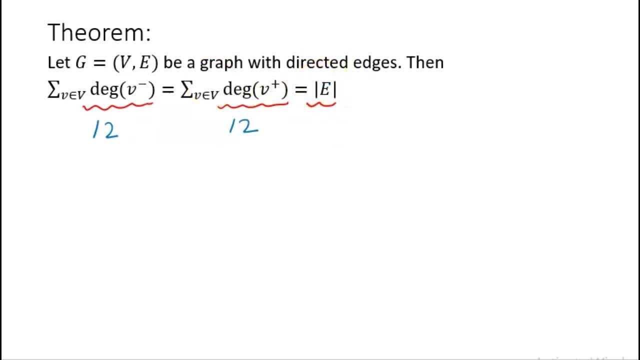 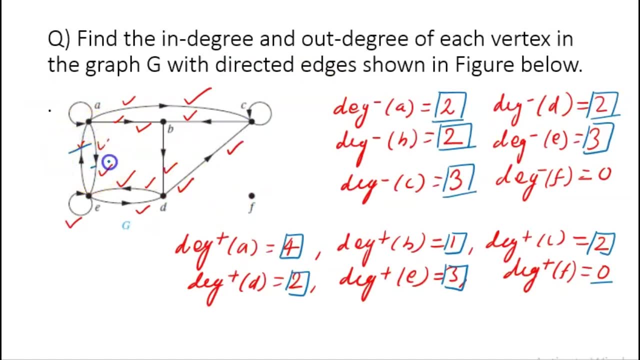 And it should be equal to the number of edges present in the graph. So let us verify it. How many edges are present? So let us count them: 1 edge, 2 edge, 3 edge- this is also an edge- 4 edge, 5 edge, 6 edge, 7,, 8,, 9,, 10,, 11 and 12.. 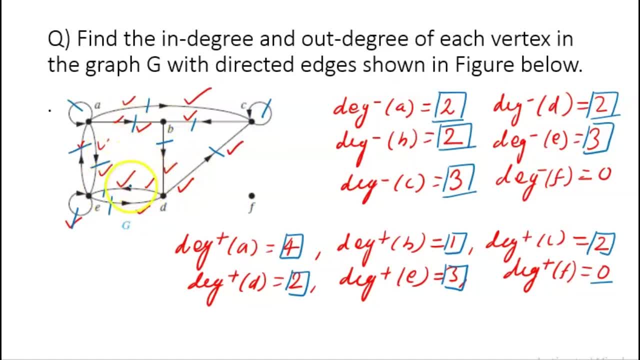 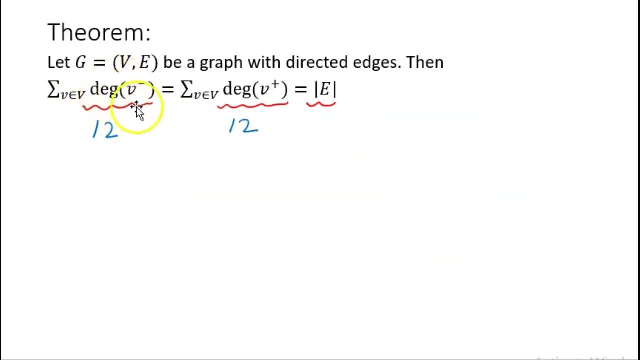 So how many edges are there? There are 12 edges and the theorem tells us that, if I take any directed graph, the sum of its in-degrees of all its vertices is equal to sum of out-degrees of all its vertices is equal to the number of edges present in the graph. 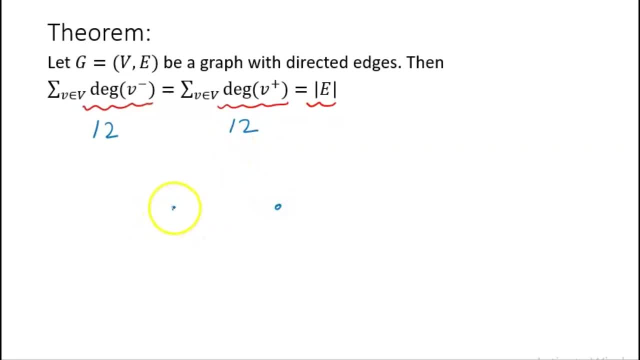 Just to verify. let us quickly. you know, and I think you can verify it yourself, You can draw any random directed graph and verify that if you take the sum of the in-degrees of all the vertices present in the graph and sum of out-degrees present in